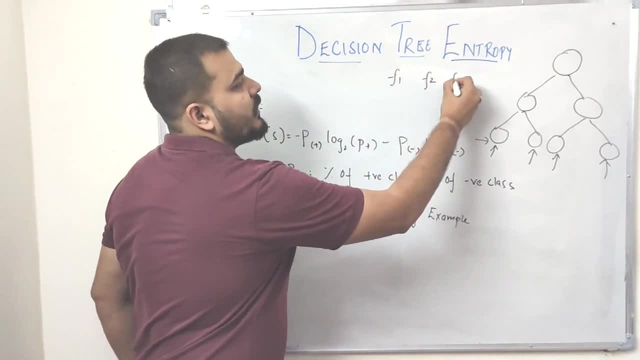 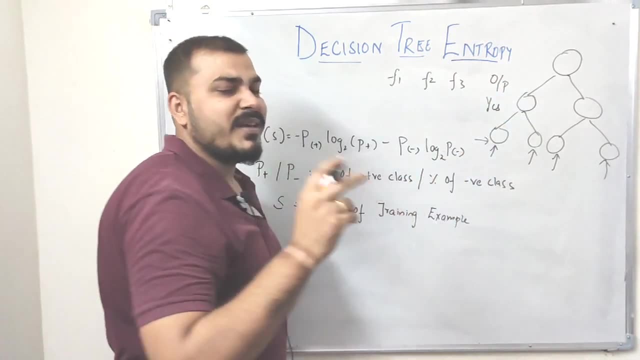 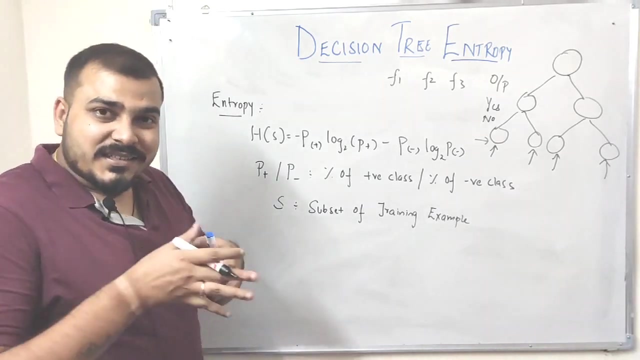 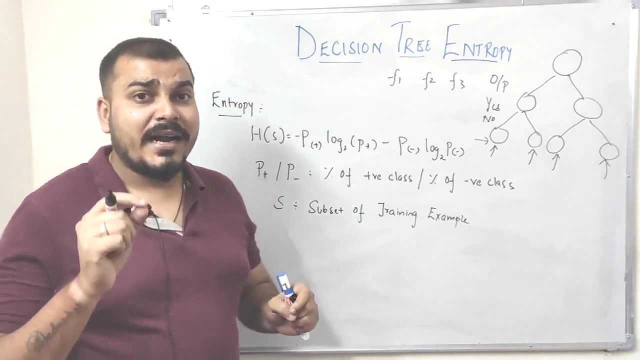 Suppose I have feature F1,, F2, F3 and, based on this feature, I have a dependent feature which is like output, and the type of output is basically a binary classification, So the output will be either yes or no. Okay, Now, while constructing the decision tree, there is a concept or there is an algorithm which is called as ID3 algorithm. The ID3 algorithm basically says that the first step is to select the right attribute for the split tree. 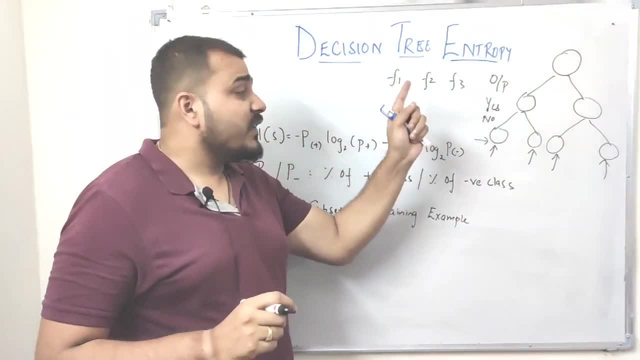 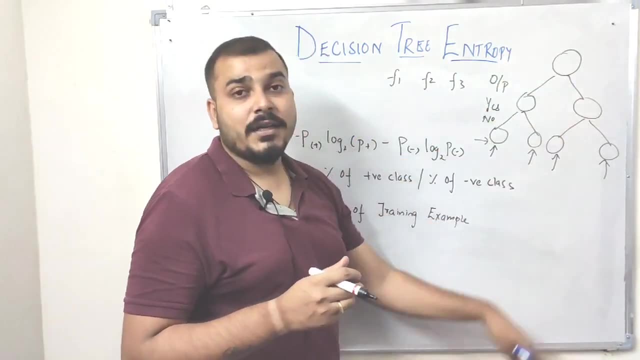 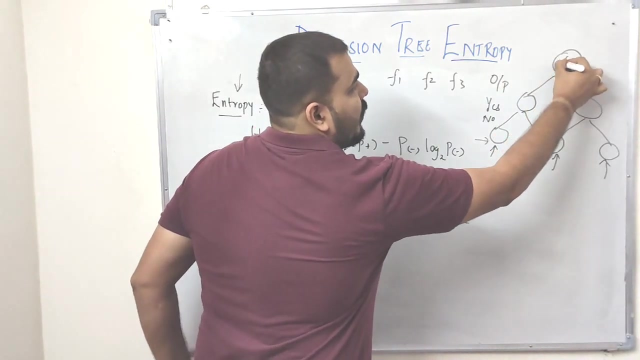 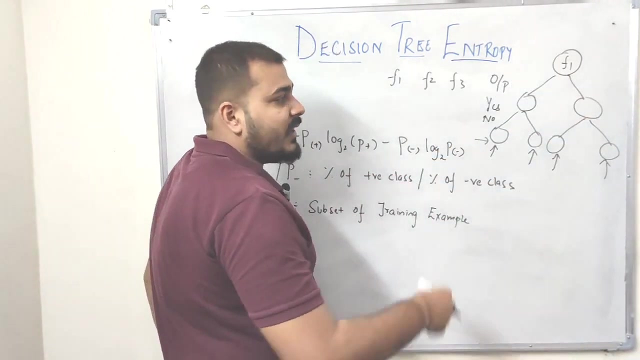 Which is the first feature that I should consider as a node. So, in order to consider which feature should I use for splitting the nodes, that basically means that we have to use this entropy technique Because, remember, guys, suppose I am considering this F1 node Right Now. based on the categories inside my F1, which is my this feature- I will be splitting these nodes And then, after this, I may select F2 node, Then I may select F3 node over here. 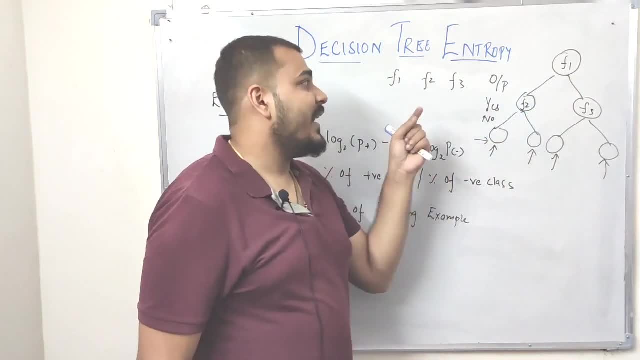 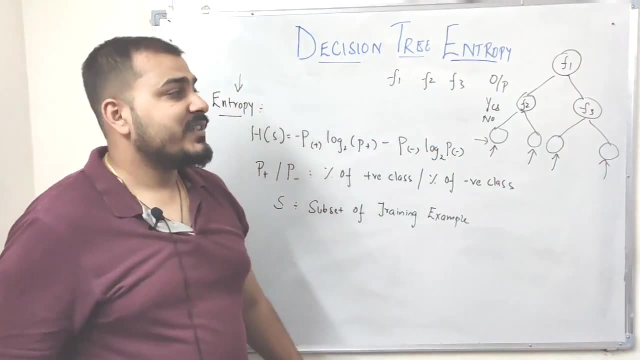 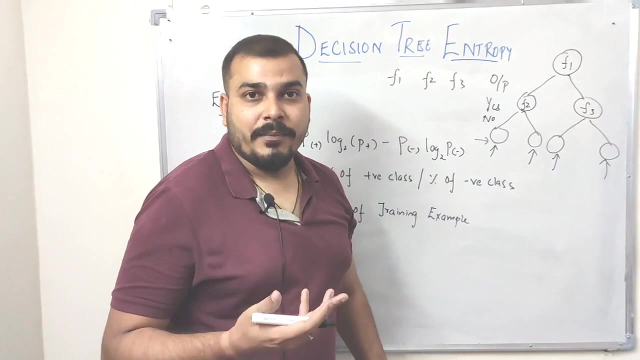 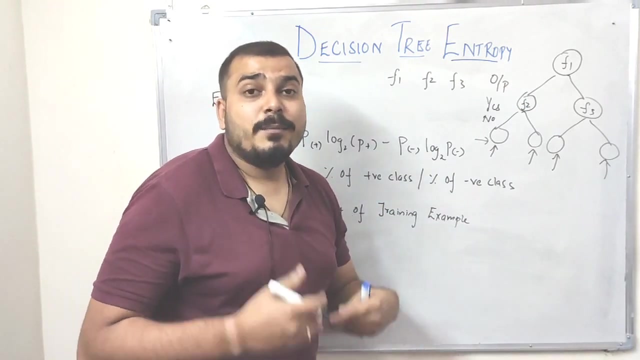 Right. So we should understand how should we select the right attribute? We can also proceed with F2 over here Or F3 over here, Right? So what is the basic approach to select the right attribute for the splitting purpose? Because if I select it in the right way, I may get the leaf node very quickly. Otherwise, if I don't select this, then my division of the tree may go till much depth, You know, And it may take much time. So, in order to see that, to select the best attribute of the node, 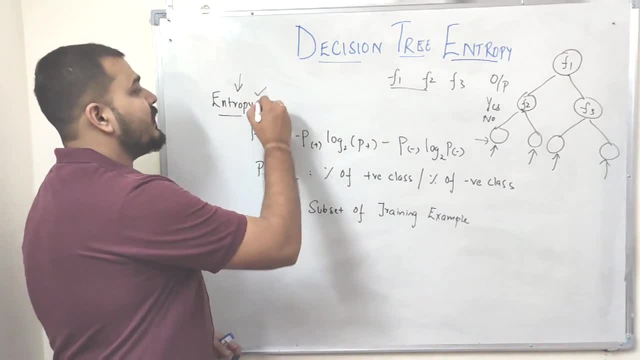 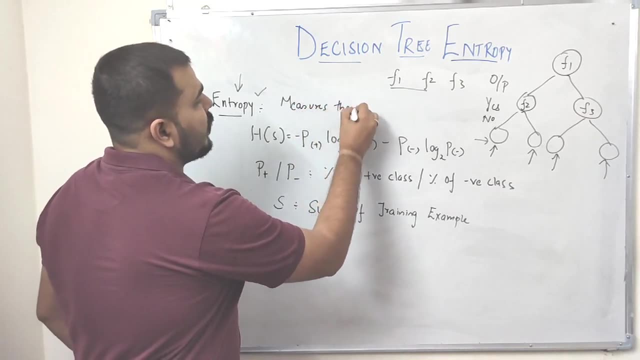 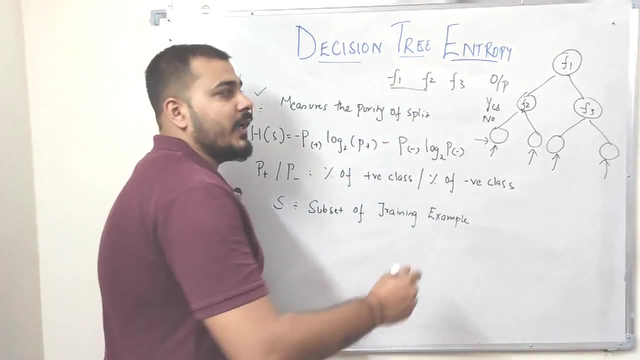 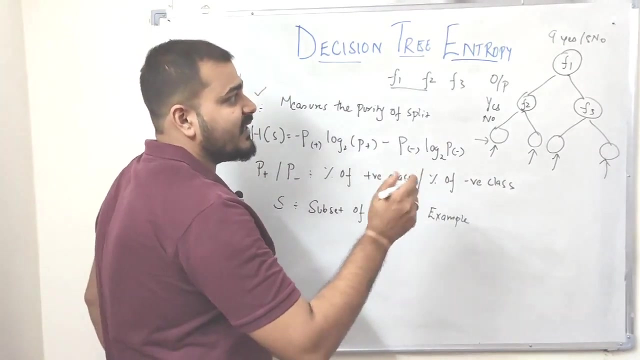 So this is the best attribute in case of the feature which basically applies something called as entropy. Now, entropy helps us to measure the purity of the split, Measures the purity of the split. Now understand guys. Suppose I selected F1. Initially I had 9 yes and 5 no's, And this is basically my output class labels. So I am basically saying that 9 records says 9 yes And remaining 5 records had no's and no's. 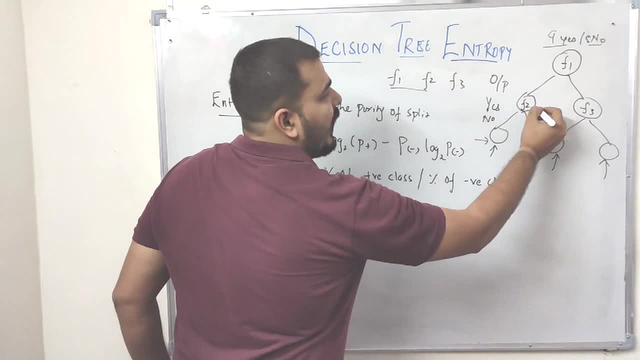 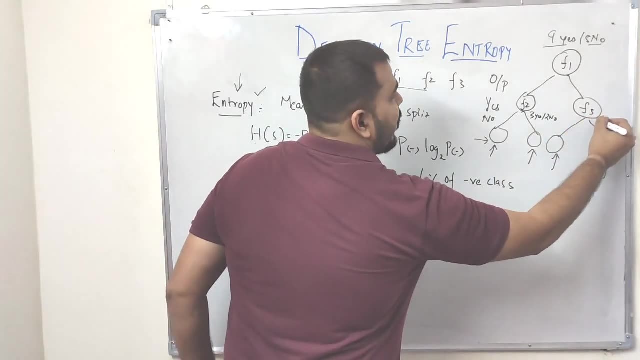 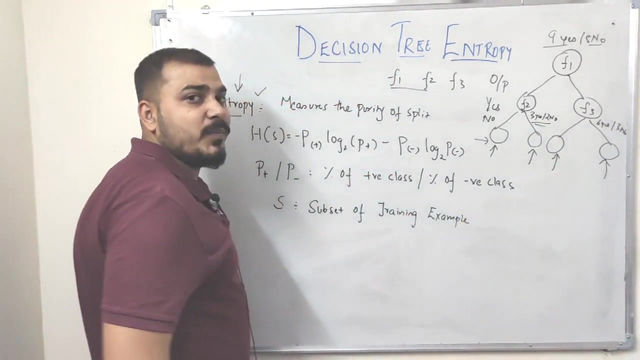 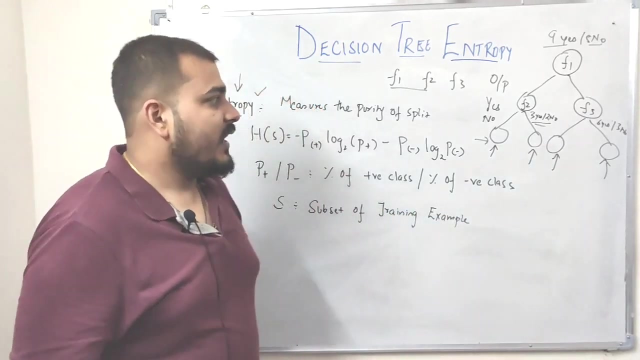 As its output. Okay, But after I selected F2, I got somewhere around 3 yes and 2 no's, And in this case, suppose, I got somewhere around 6 yes and 3 no's. Now you can see over here this is not a pure sub-split, Because pure sub-split basically means that either you should be getting yes or you should be getting no. Okay. So again, what I did is that, based on this F2, I took it and I started splitting more. 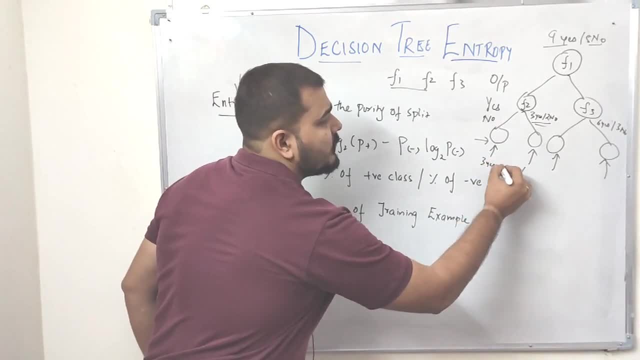 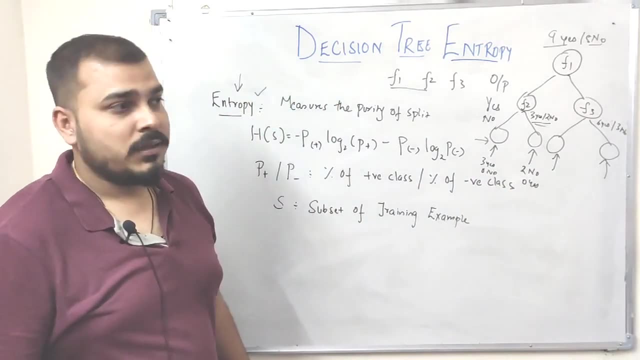 And suppose in this case I got 3 yes and 0 no's as my output. And here I got 0 no's and 0 yes, Sorry, 2 no's and 0 yes. Now, here you can see, I have got a pure sub-split In this particular case. whenever my branch happens to this particular path, at that time I am also going to get always the output as yes. This is basically my leaf node. And similarly in this case, suppose I get 6 yes here and 3 no's over here, Right, This is basically my leaf node. 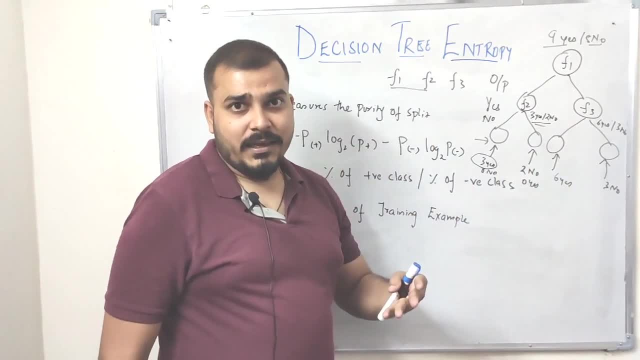 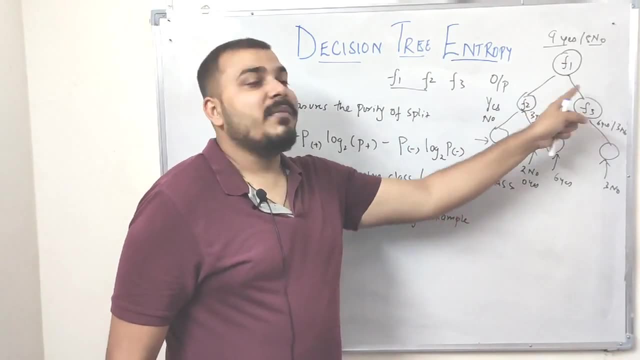 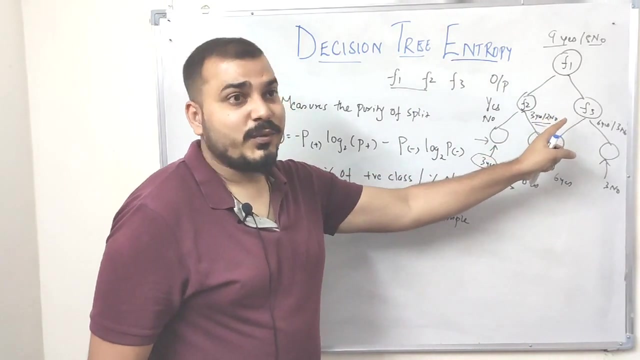 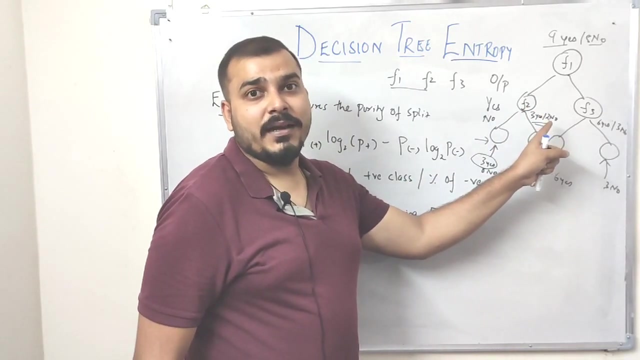 Now, in order to get the leaf node quickly- and we should do that, we should aim in a decision tree that we should be able to get the leaf node quickly- We have to select the right parameters. These parameters are basically my features of the data set. Okay. And in order to set this, we need to make sure that the purity split. we have to go and calculate the purity of this particular split every time in each and every node, So for that we use something called as entropy. 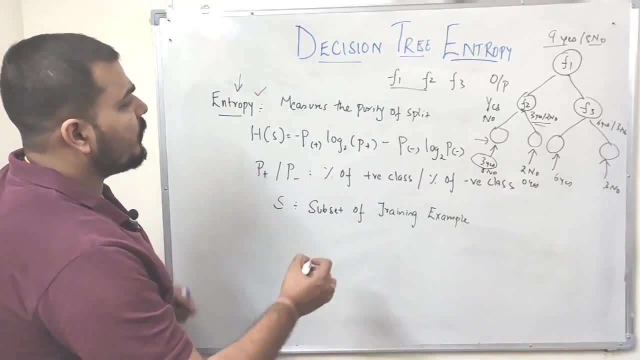 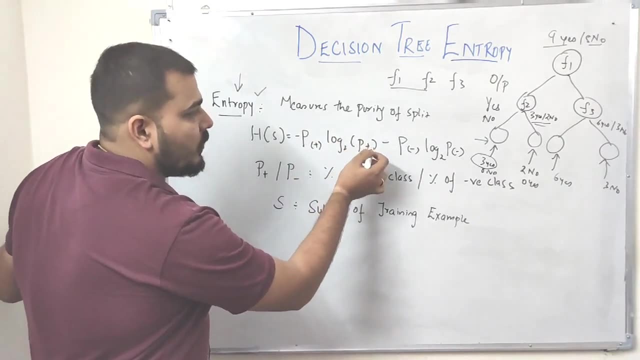 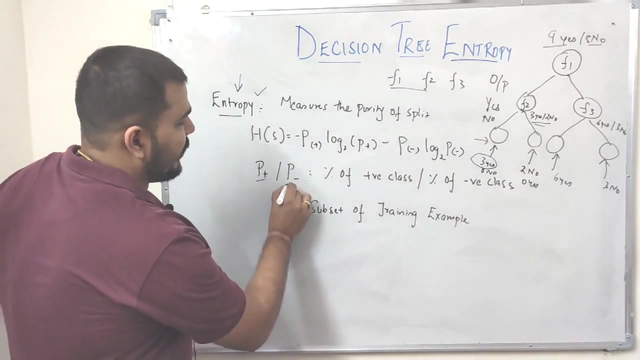 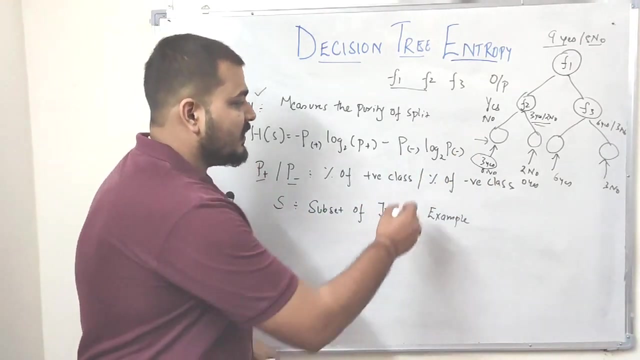 Now entropy. you can see that it measures the purity of the split And the formula is simple: Minus probability of plus. I will say you this probability of plus means what? Log of base 2 probability of plus. minus. probability of negative. log of base 2 probability of negative. Okay, Now, what does this P plus and P minus say? It says that percentage of positive class divided by percentage of negative class. Okay, This divided is just like I am saying that, or P negative is basically percentage of negative class. 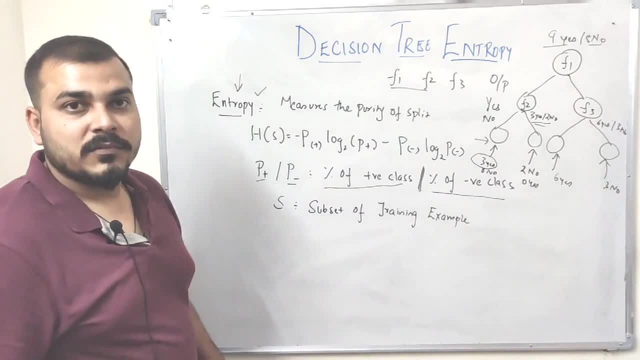 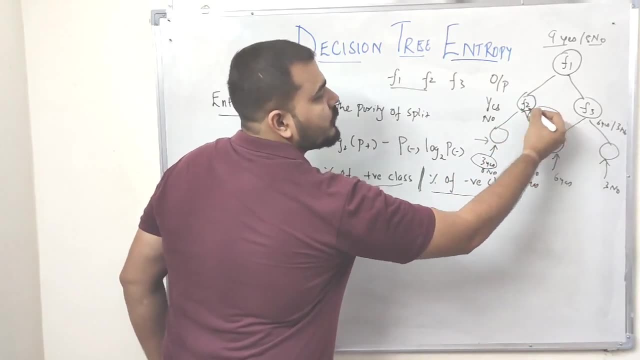 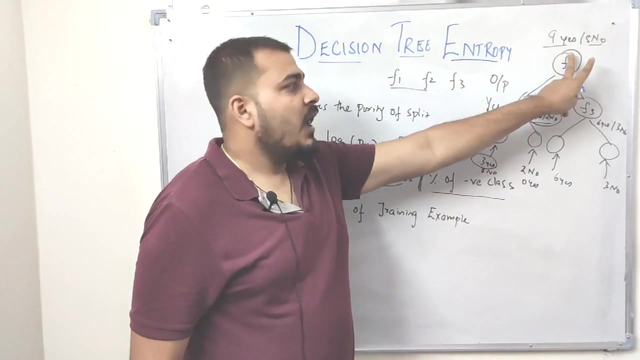 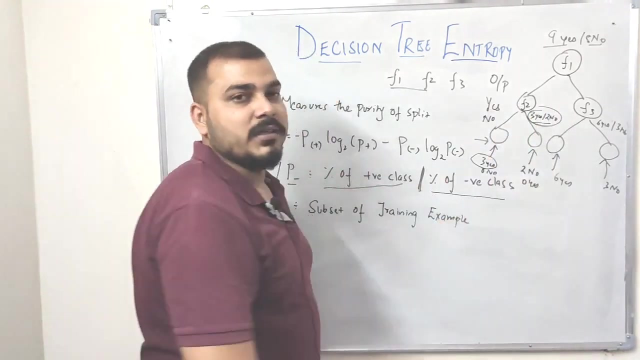 P positive is nothing but percentage of positive class. Now you do understand that. Now what is this positive class? Now just imagine, guys, after this split I got 3 yes and 2 no's, Right? If I want to calculate the entropy of this particular node, Suppose I have selected this particular node. After this I want to decide whether I have to go with F2 or F3 for the first splitting. So I will go and compute the entropy of both this And entropy. in this case, I have 3 yes and 2 no's and 6 yes and 3 no's, Right. 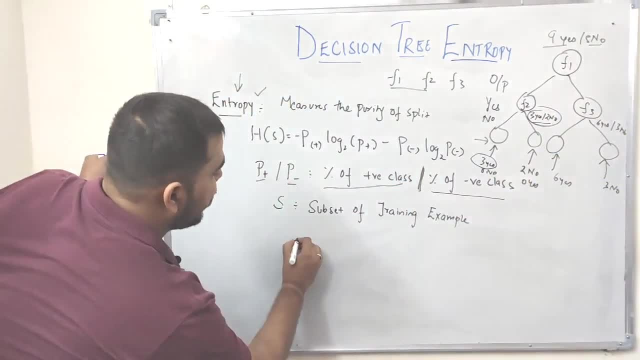 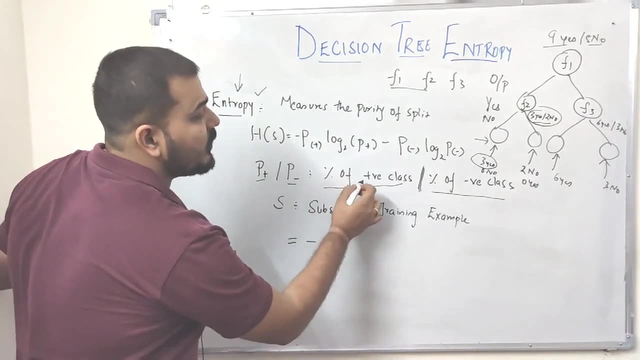 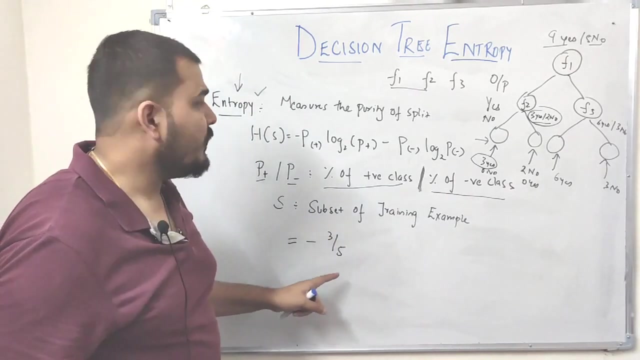 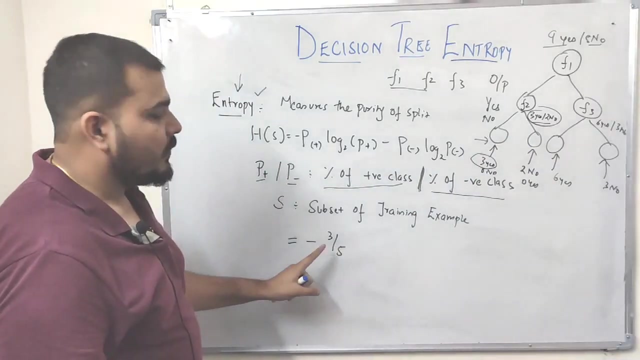 So let me just calculate the entropy of this Now, entropy over here. I can write it as. Understand this formula: Negative and probability of plus, This is nothing but percentage of positive class. You can see that I have 3, yes, divided by 5.. Why I am taking 5? Because since I have to calculate the percent in the denominator, I have to take the whole number of records, Right. So it is like 3 by 5.. And again, I have log base: 2, 3 by 5.. 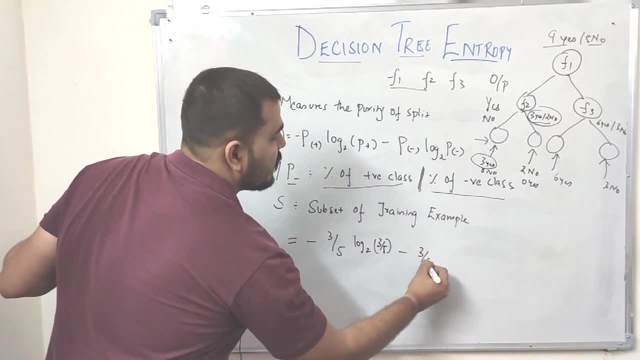 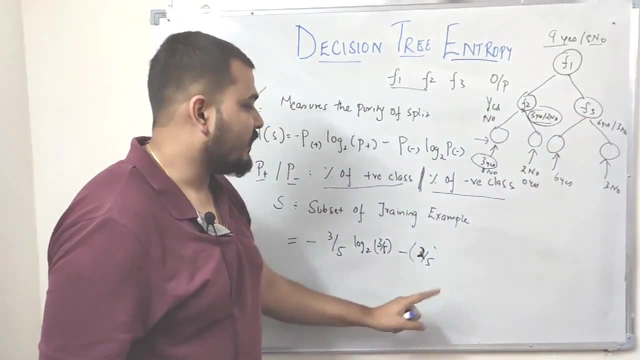 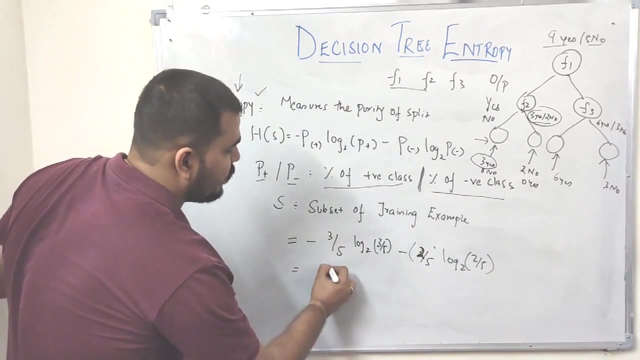 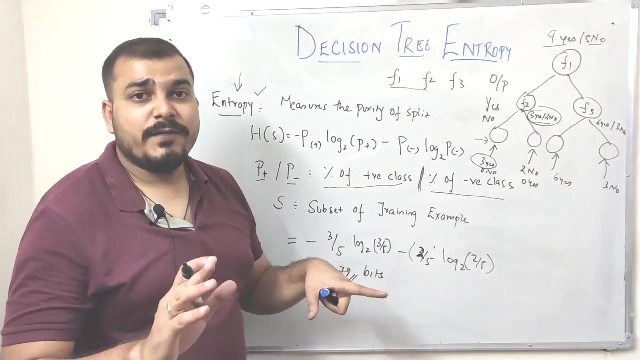 Minus, Priority of minus, What is probability of minus? 3 by 5? again, Sorry, this is 2 by 5.. Because I have 2 no's and total number of records are 5 and log of base: 2, 2 by 5.. Now when I compute it I may get somewhere around, you know, 0.78.. 0.78 bits. And always remember, guys, if you have a complete impure subset. Complete impure subset basically means like this: 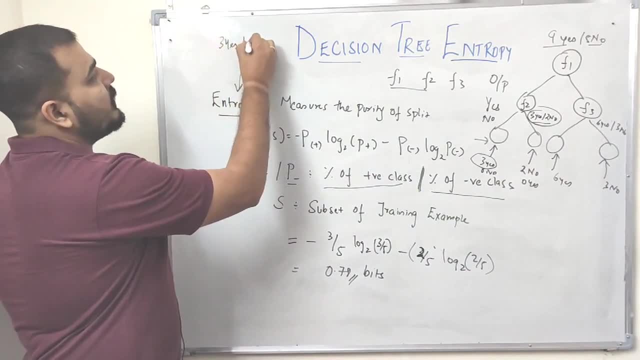 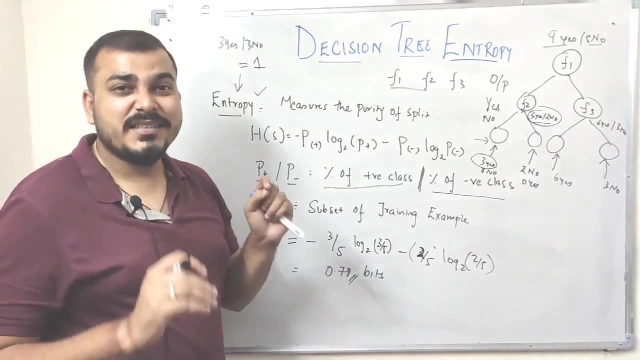 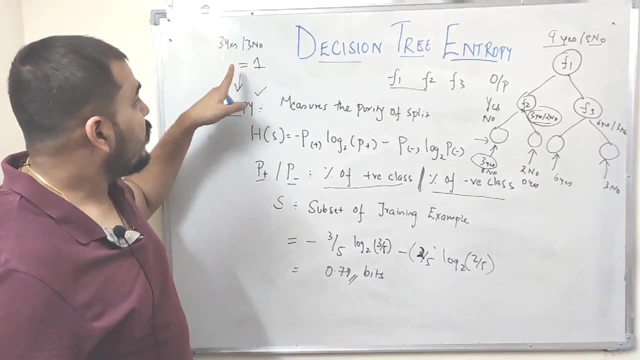 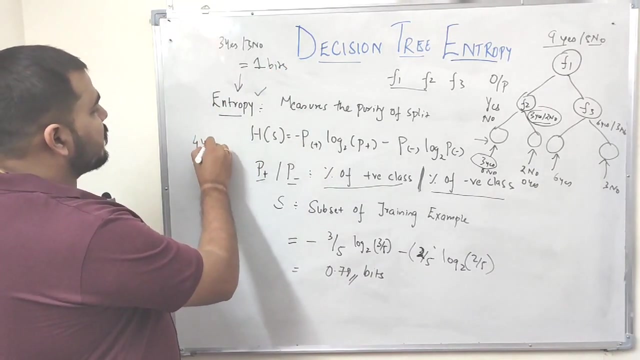 Suppose you have a scenario where you have 3 yes and 3 no's. In this scenario, your entropy will always be 1.. This is the worst split Because it is completely impure. You have 50% of probability saying it yes, 50% of probability saying it no. Right, So it will be basically 1 bit. And always remember, for a pure soft split, Suppose I have a case wherein I have 4 yes and 0 no's. For this, if I try to compute in this, I will definitely get it as 0 bit. 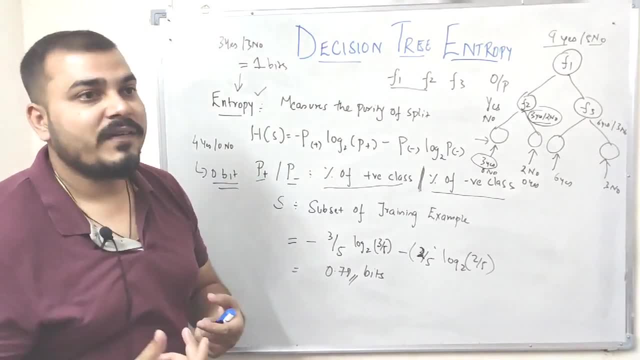 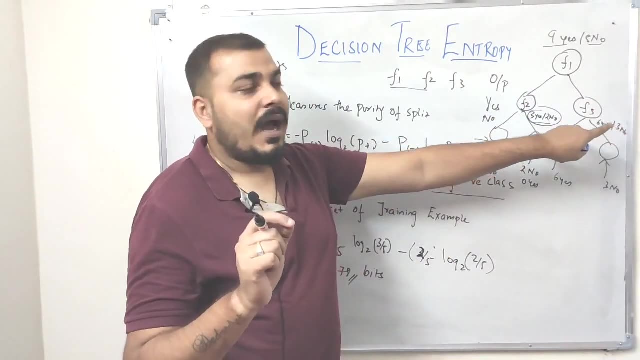 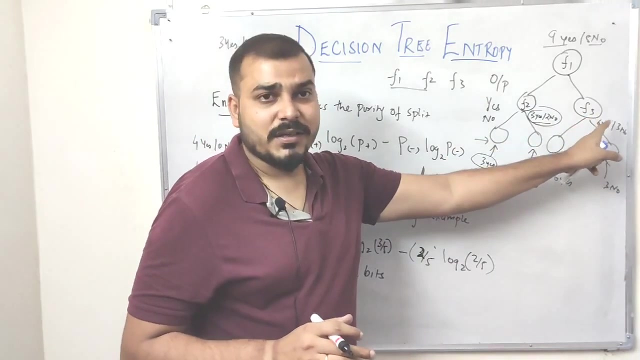 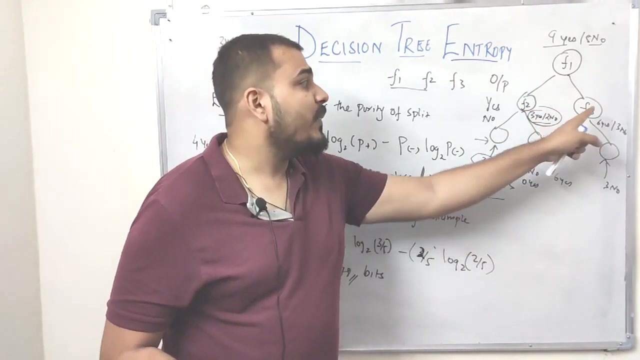 So you should understand that the entropy of the value is between 0 to 1.. Now what I do is that suppose I want to select F2 or F3 first. I will go and compute the entropy of this. Okay, If I get the entropy lesser in the lesser value and compared to this, Suppose this particular entropy is 0.75.. This particular entropy is 0.5.. That basically means that this entropy value is much more better than that. So I may go ahead and select F2 and start splitting it, Okay. 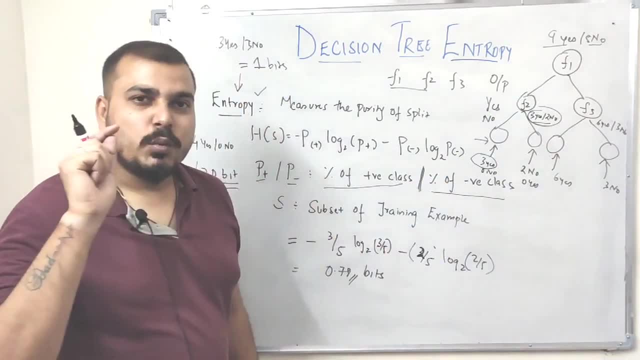 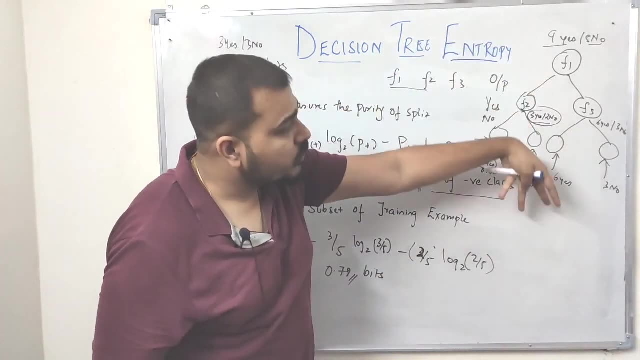 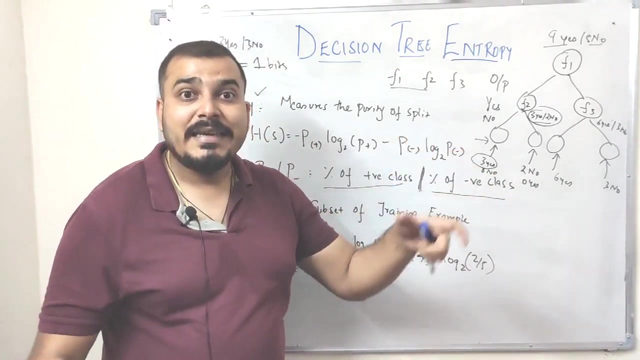 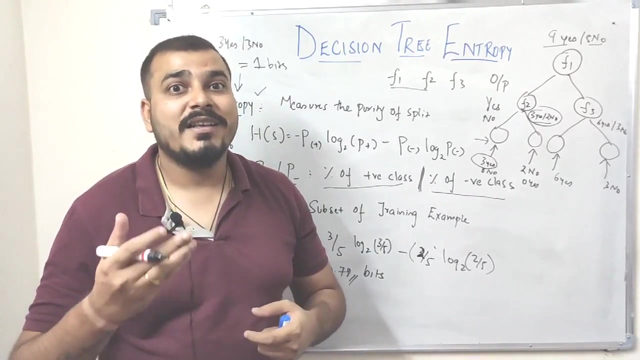 But understand, guys, This. I am talking with respect to just one node, Right, But we should also consider, after I split this, I may also require some other attributes to reach the leaf node, And I also have to take the entropy of those values and add it up Do the summation of all those entropy values. So for that we have a new concept called as information gain. Information gain makes sure that from the top till the end, 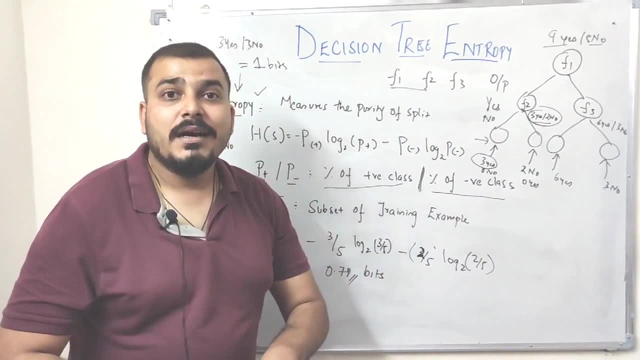 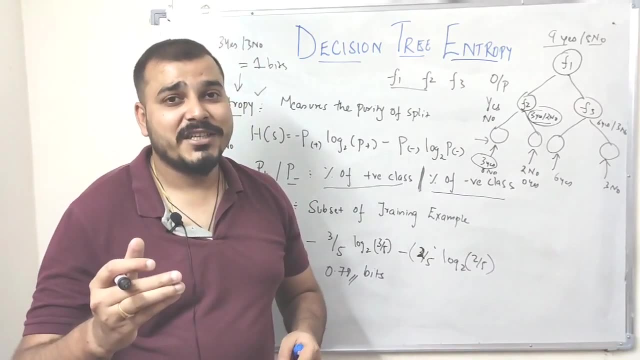 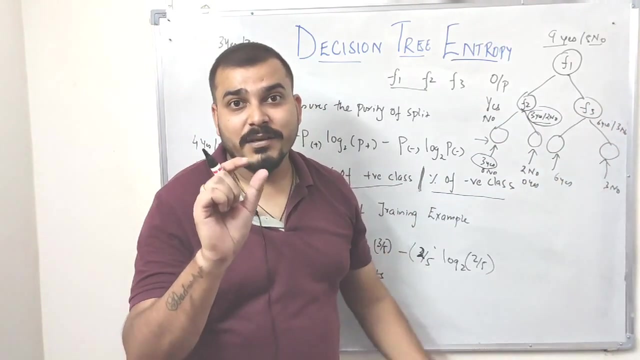 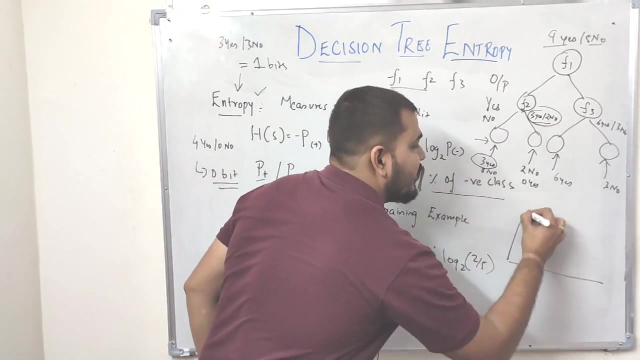 Till the leaf node. It will go and compute what is a very good entropy value, What is the total entropy value, Along with some different formula which I will be discussing about information gain in my next session, In my next video. But this particular video is more focused with respect to single, single nodes. And always remember, guys, Entropy values ranges between 0 to 1.. Okay. Now, when I say 0 to 1, it will be looking something like this: This is the 0. This is the 1.. Okay, And entropy value always ranges between 0 to 1. Okay. 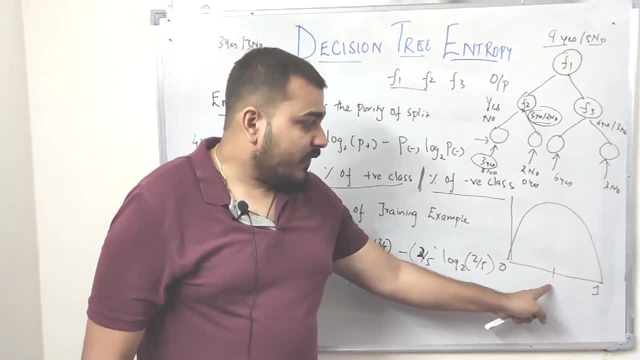 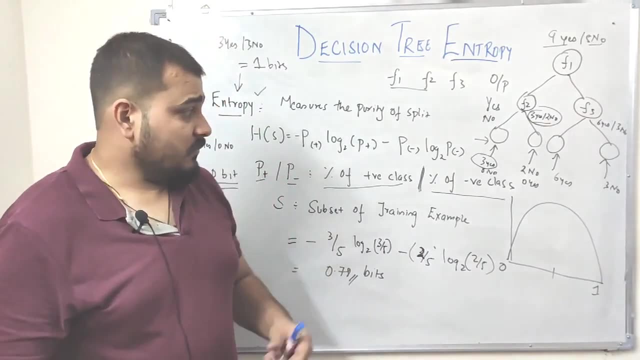 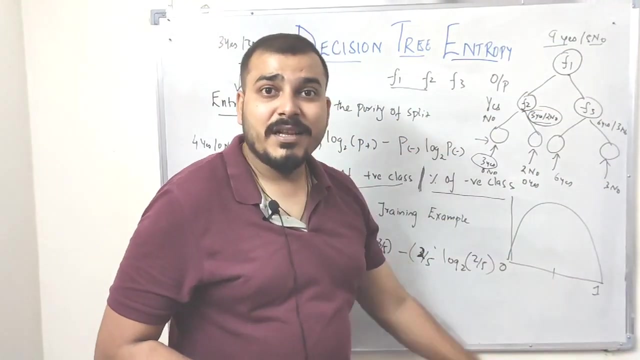 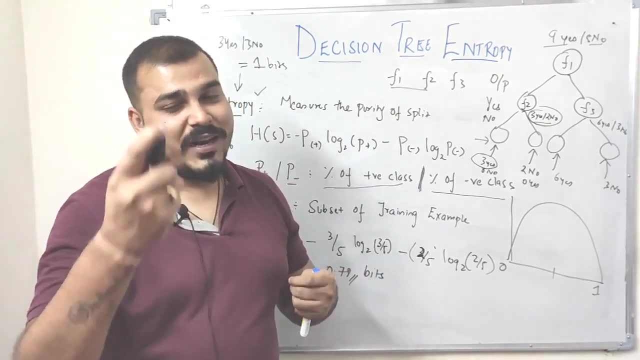 So if it is 1. That basically means it is a completely impure subset. So in my next video I will be explaining about information gain, Because entropy is just calculated for one node. If you want to calculate the information, I mean the entropy of all the nodes, till the depth, till the leaf node- We basically use information gain. Information gain combines all the entropy together And I will just show you that formula in my next session, Because that will also be a very simple formula And that is what it happens. 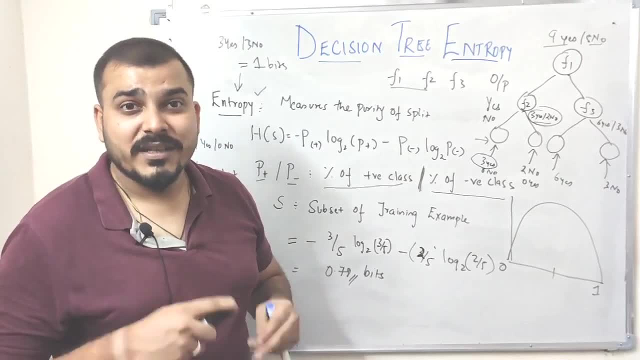 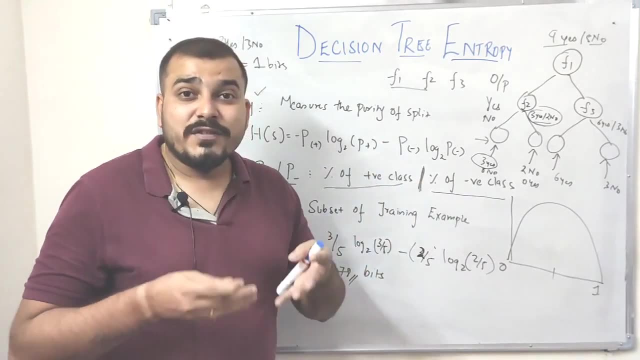 in each and every algorithm. whenever we are applying decision tree with respect to any data set that we want, We will go ahead and calculate the entropy and we will try to find out which feature is best for splitting it, and then we get the whole decision tree that. 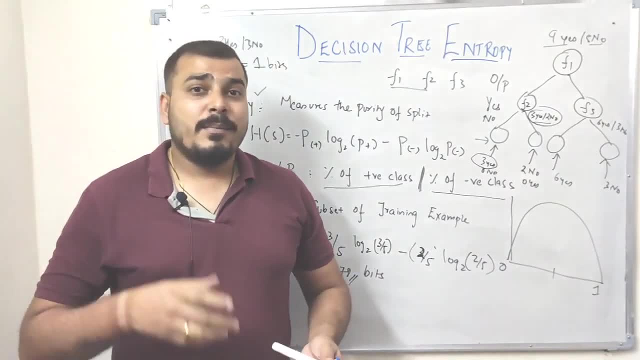 is basically created, So I will see you all in the next video. Have a great day ahead. Please do subscribe the channel If you have not already subscribed. I will meet you all in the next video. Thank you one and all. God bless you.